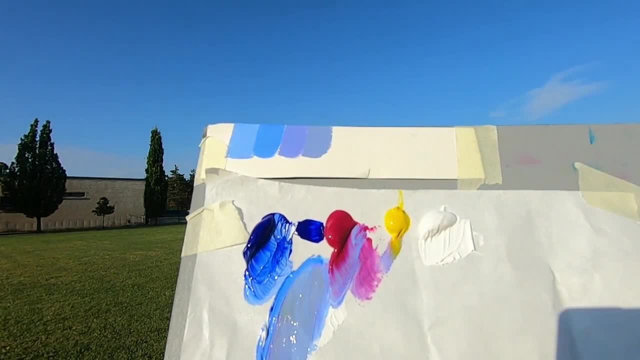 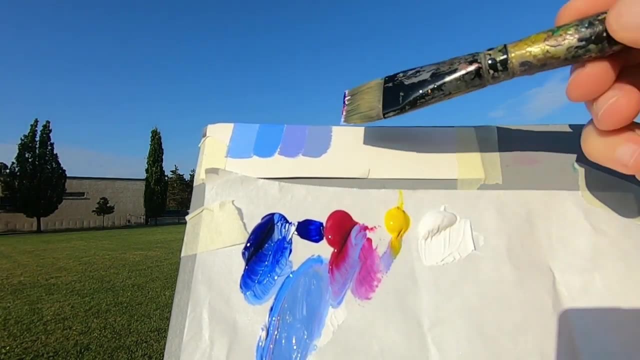 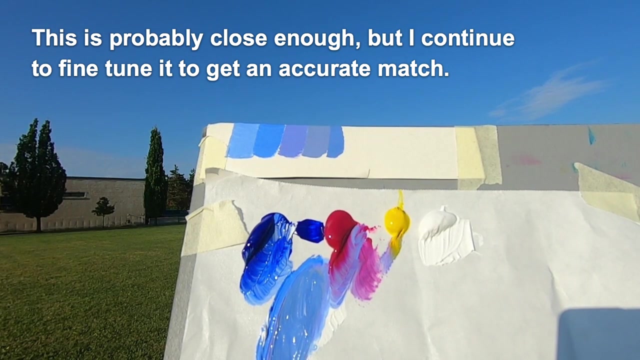 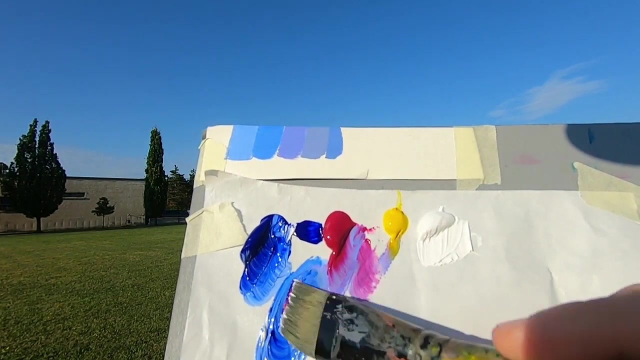 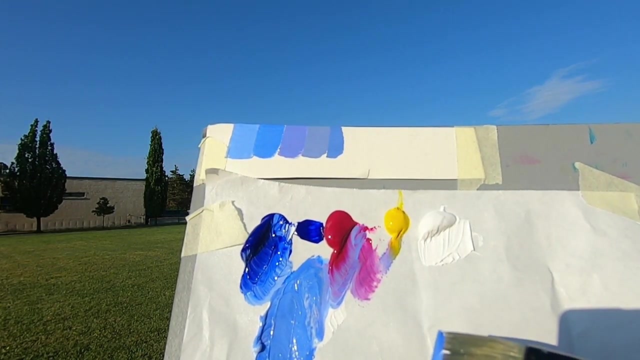 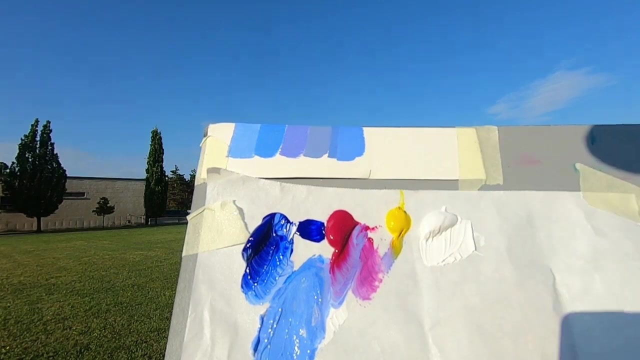 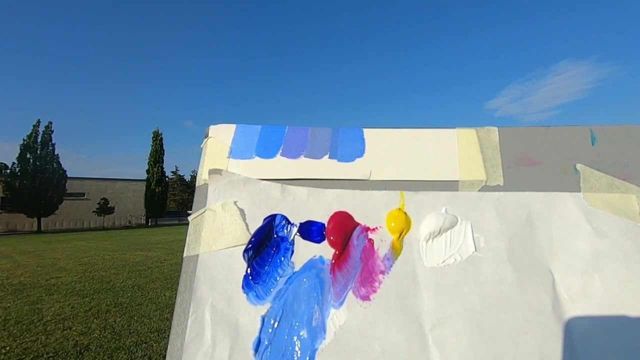 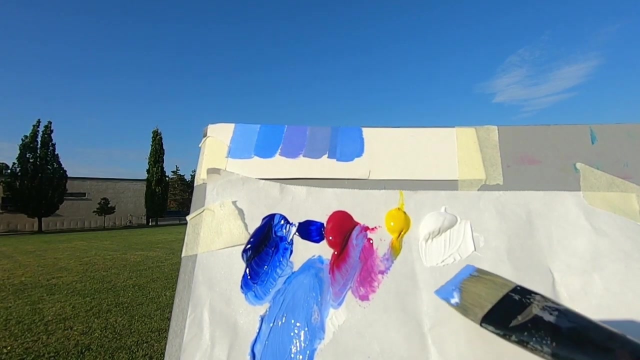 Okay, I think it needs more blue. Getting there, I think more blue. There comes a big garbage truck. How many times is that thing going to back up? Okay, he's dumping the garbage. Oh, there you go. Okay, acrylic's dry. it's slightly darker, so I'm going to add a touch more white. 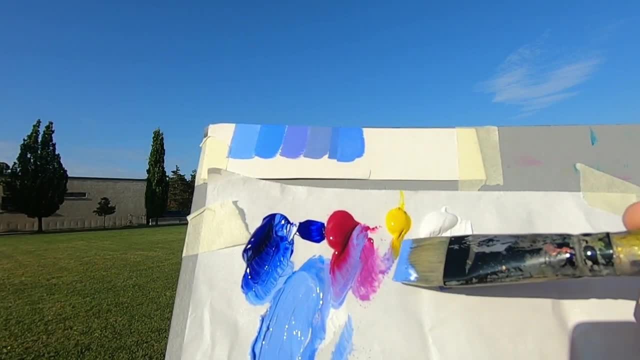 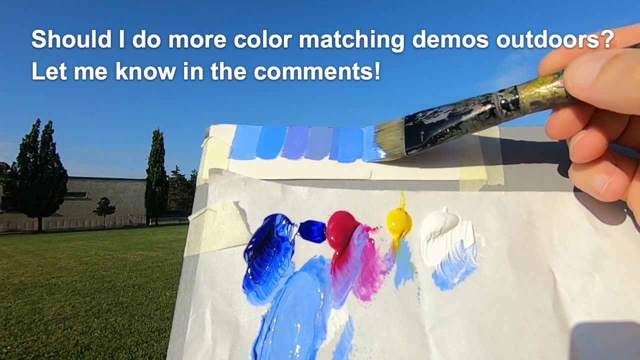 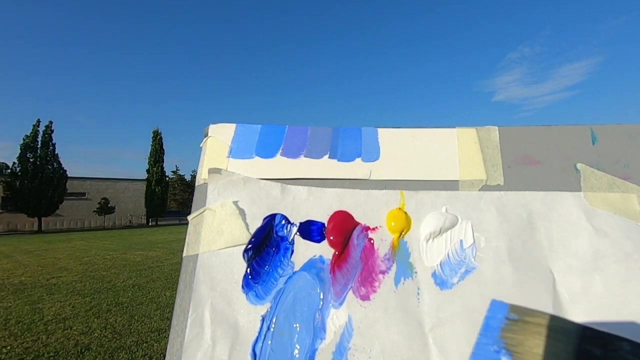 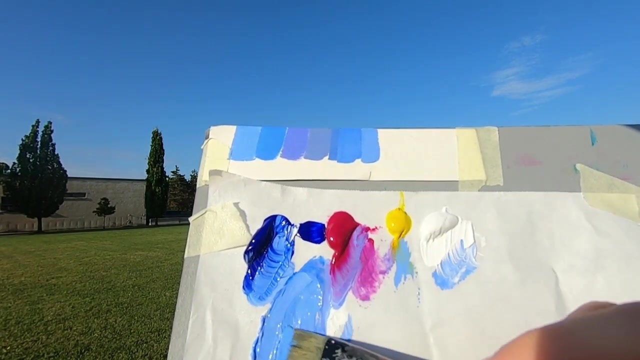 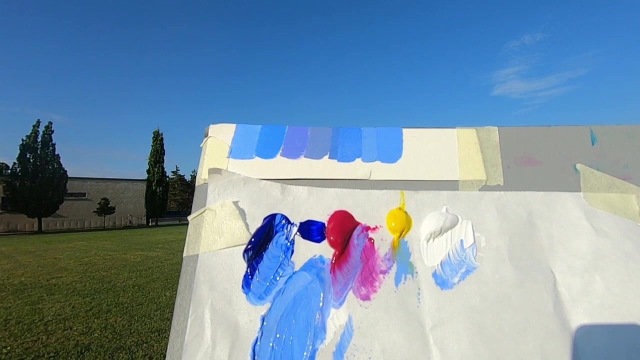 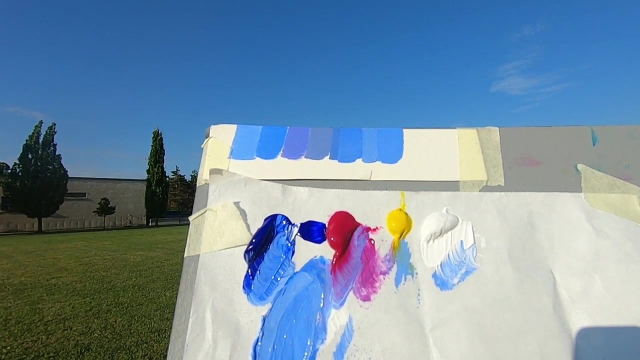 I also think just a little bit more yellow. It looks a lot lighter, but when it dries it gets darker. Maybe I want to light with that. I'd say that color's pretty close. it's just it's waiting for it to dry so I get a better gauge of how close it is. 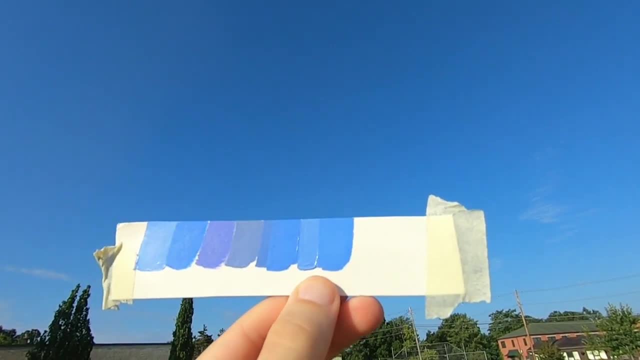 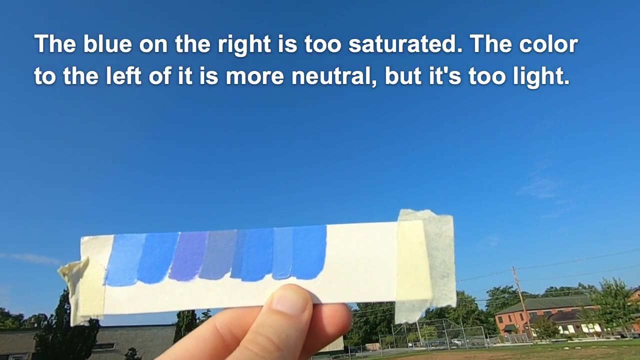 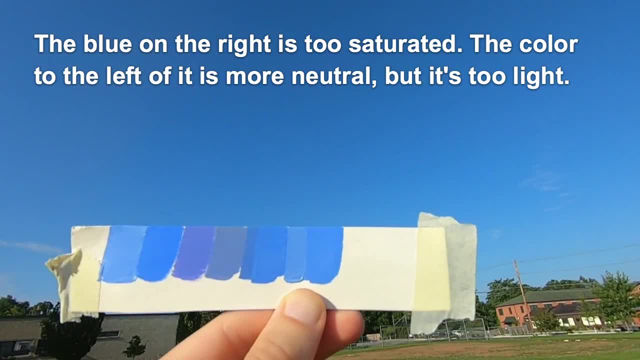 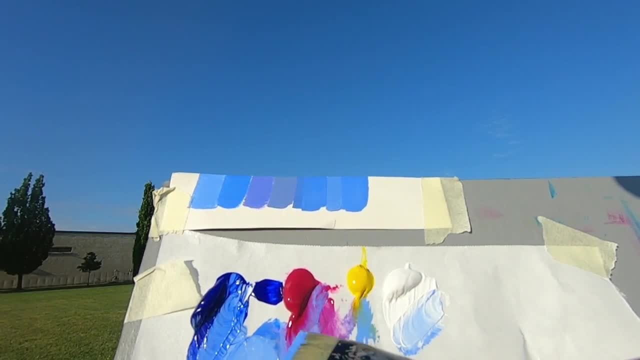